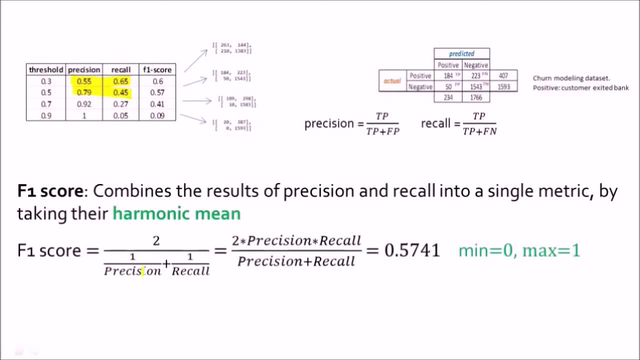 like this It is, since it is harmonic mean mean. it is one divided by precision and one divided by recall. in the denominator and in the numerator it is the number of terms in the denominator, so we have two here. so two upon these two quantities and after simplifying it becomes twice into precision, recall upon precision. 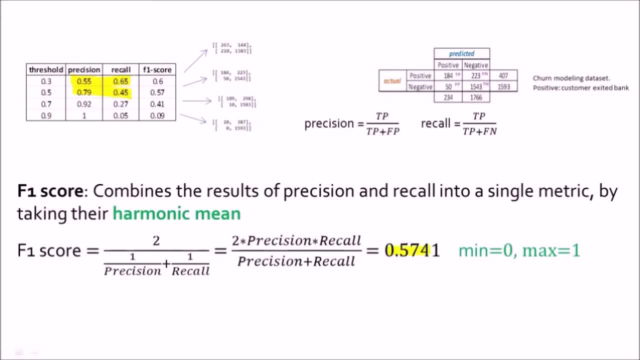 plus recall. so in our case it happens to be 0.57 for the default setting of 50 percent. now the minimum value and maximum value. the maximum can be one, of course, because if we input, precision is equal to 1 and recall is equal to 1, that is, if we have no false positives and no false negatives. 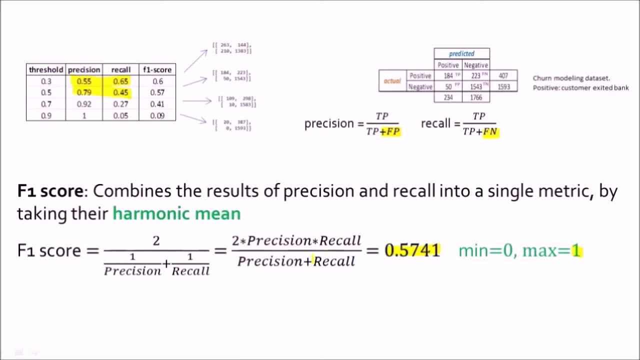 we would have precision and recall equal to 1, so our f1 score will be 1. and as for the minimum case, well, just think about it, if we have 0 precision, then we would have 1 upon 0 in the denominator here. then this would become undefined and hence, just imagine, we have a very small precision value. 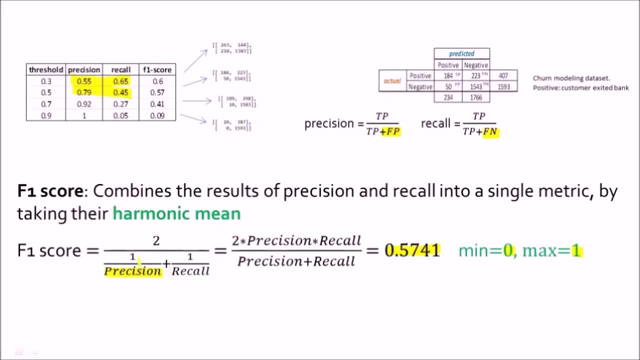 then this number will be a very huge number. 1 upon very small number is a big number and again, if we have a very small recall value, then again we would have a very big number here and big number plus big number will be a very big number. and 2 divided by a very big number. 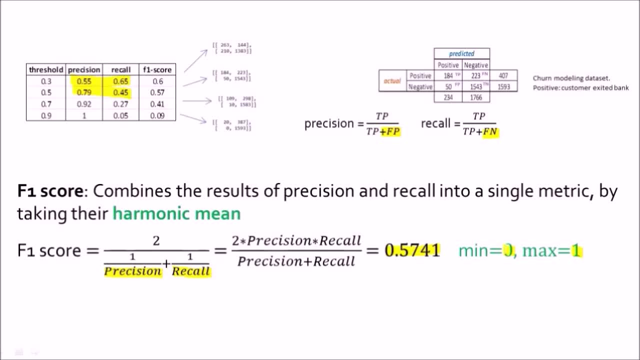 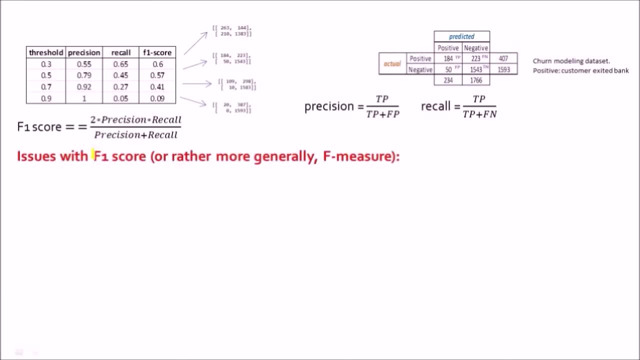 will be a very small number and hence the minimum can be approximated towards 0. now there are a few issues with the implementation of f score or f1 score. now, this f1 score is just one of the family members of this bigger f measure family. now, first issue is that the f1 score gives equal importance. 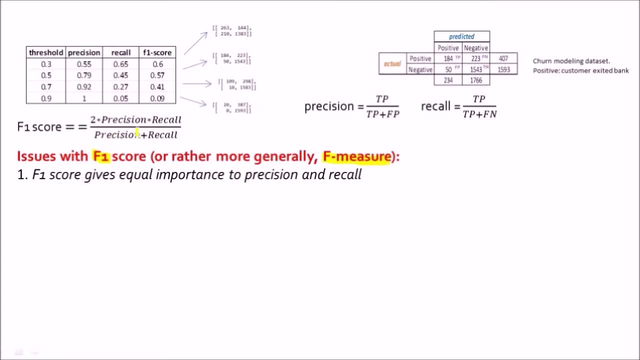 to precision and recall. if we look at the formula, we notice that it is giving equal importance to both precision and recall, which is a source of some criticism, because in different real life scenarios the cost of false positives and false negatives are different and we cannot equate. 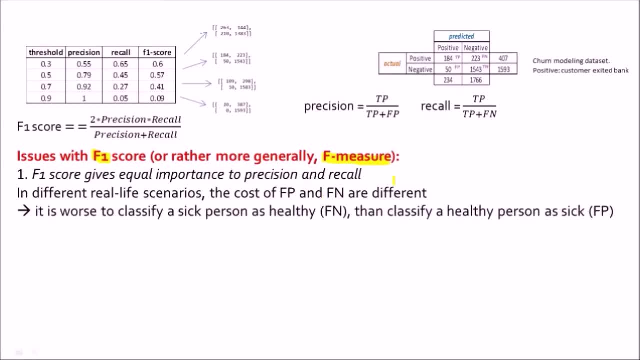 false positives to be equal to false negatives. for example, it is worse to classify a sick person as healthy, which is a false negative case, than classify a healthy person as sick, which is a false positive case. right, because if you classify a sick person as healthy, then they would not get any further treatment done or they wouldn't take. 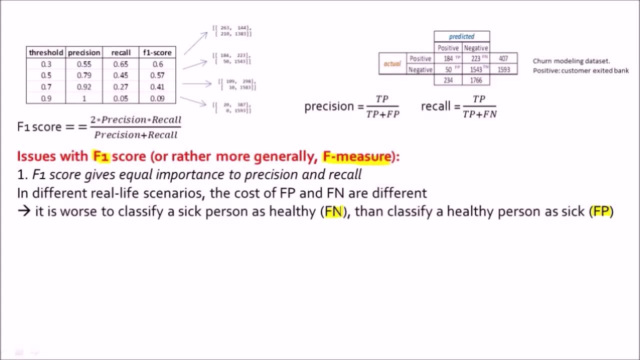 any further medications and that would be bad for their health. so that is a very bad scenario and that is a very bad classifier and if you look at the formula, false negatives is with the recall and hence, if we have a very high number of false negatives, that would mean we have a very low 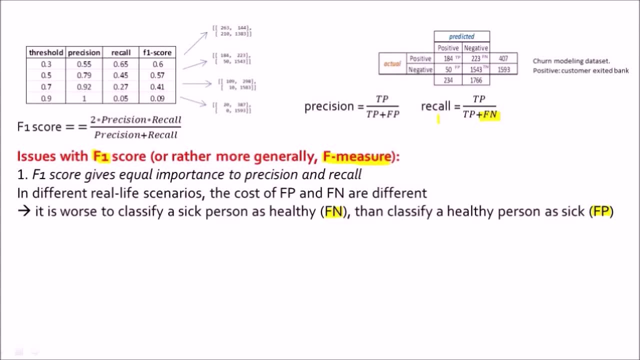 recall, and having a low recall would straight away tell us that that the classifier is not doing a good job. the second issue is that f measures in general are asymmetric. now, this first issue was only with the f1 score, because we will rectify this issue of equal. 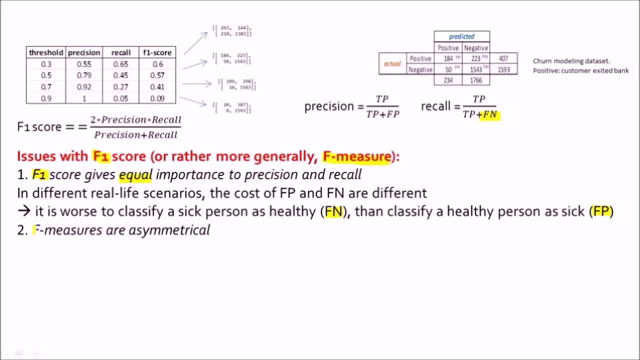 importance in the f beta measures. the second issue is the is with the whole family of f measures. so what i mean by that is if we invert the positive and negative class labels, then the results will be different. this can be a problematic issue while trying to predict apples and oranges. 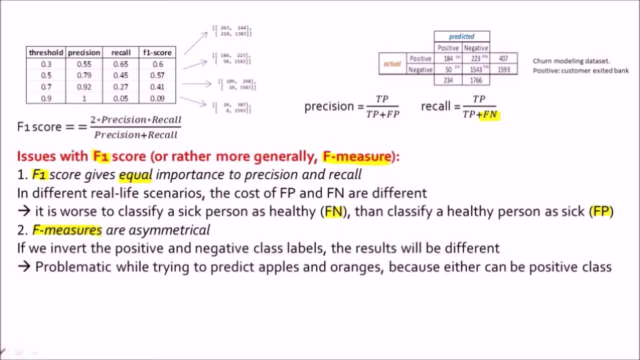 because either of them can be the positive class, right? you cannot say apples are positive and oranges or negative, always you can also say oranges are positive and apples are negative. so when you try for both of these scenarios, you will get different f1 scores and hence it would be difficult to interpret the results correctly. the third is: 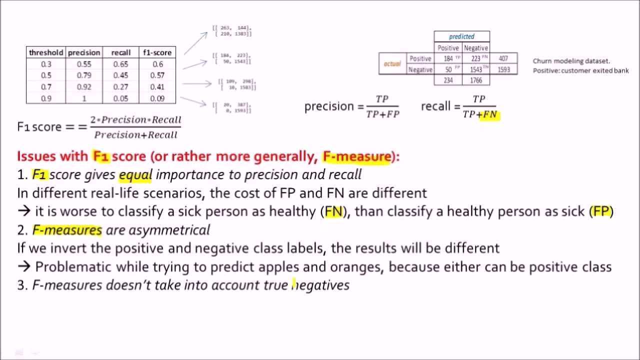 that f measures, the family of f measures, do not take into account the true negatives. so if you look at the formula for precision and recall, precision has true positive and false positive and recall has true positive and false negative, so neither of these two take it really seriously. if you look at the hundred count black hole too, it is actually true positive, as when f1, f3. 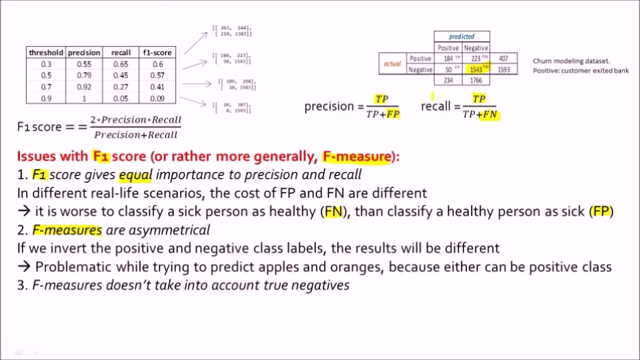 account the number of true negatives. right and since precision and recall, they form the building blocks for the f1 score. even f1 score doesn't take into account the true negatives and this can be a problem because imagine we have 100 people and 80 of them are sick and 20 are healthy. 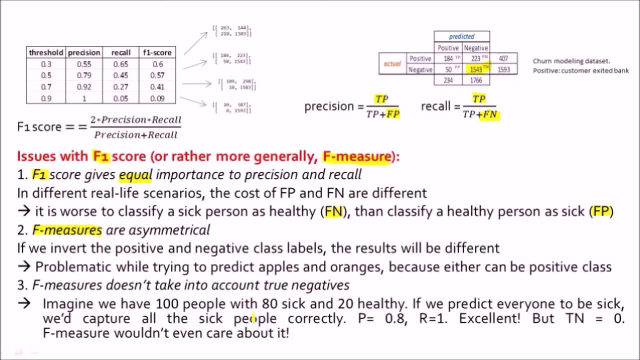 now, if you predict every single one of them to be sick, then we would definitely capture all the sick people correctly, because, since we are predicting everyone to be sick, all the 80 people will be correctly classified and if you look at the precision and recall formula, will get a precision of 0.8 and recall of 1, and if you look at the F1 score as well,